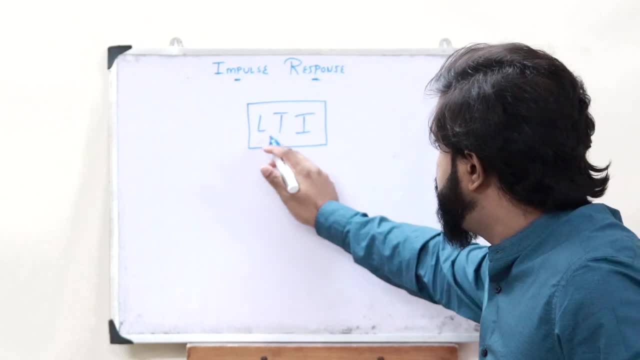 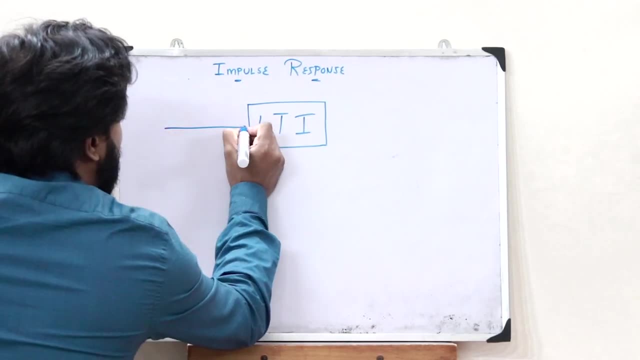 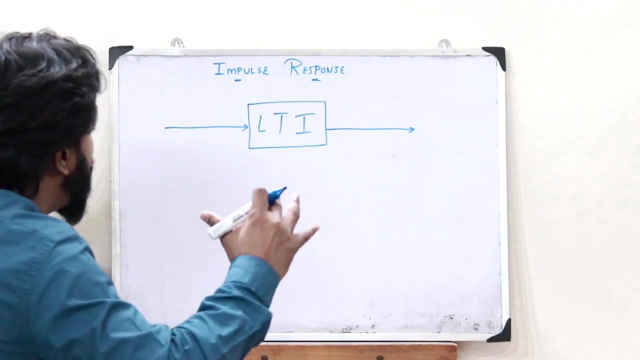 we would get what you referred to as an LTI or a linear time invariant control system. So now, here, a particular control system would have an input over here and then subsequently it would have an output over here like this, this: so now, let us assume that we are providing an impulse signal as the input to this particular 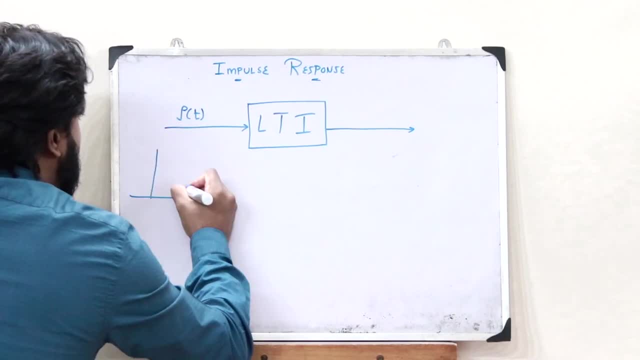 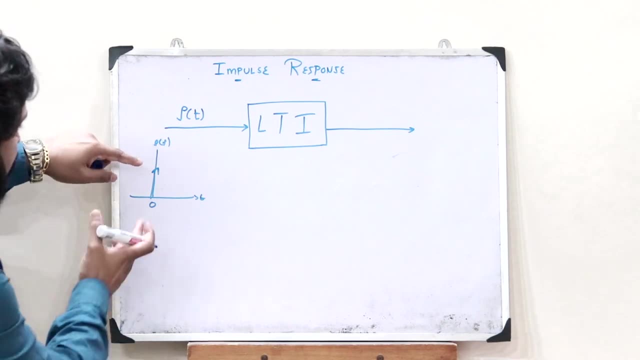 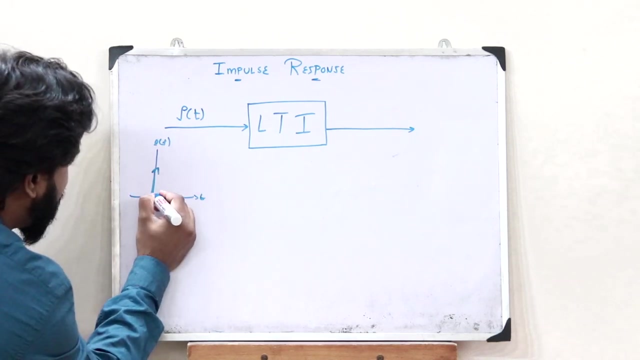 lti system. so an impulse signal would look somewhat like this. so this is an impulse signal, that is a particular signal in very small period of time. so in a very small period of time, or it would be at zero itself, so at zero itself, that is a very huge. 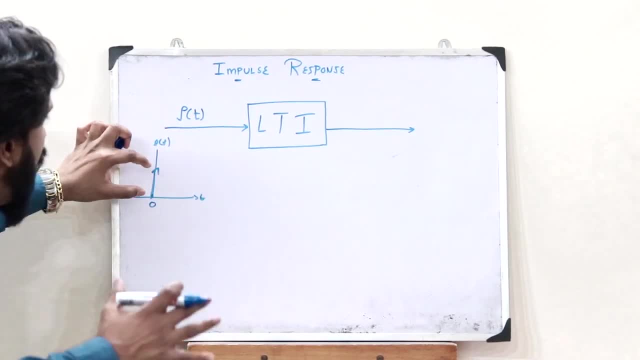 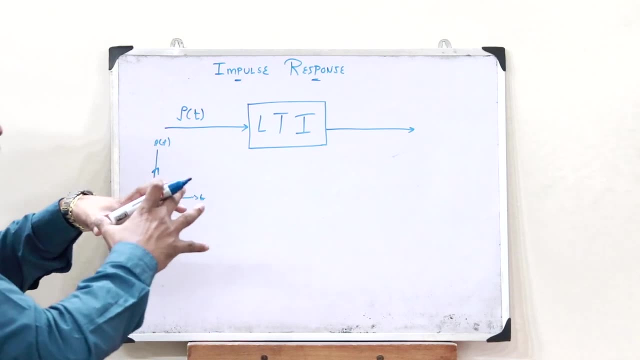 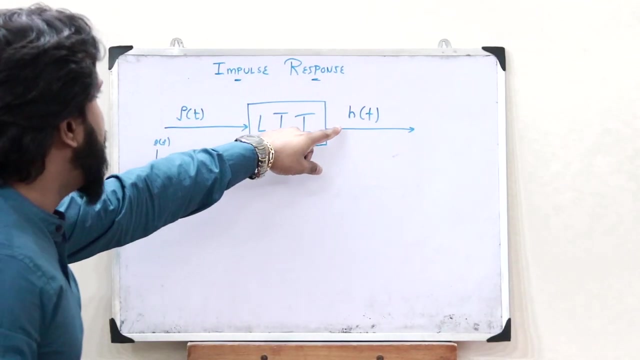 magnitude. so this is what it refers to: an impulse signal. so when this impulse signal is applied to this particular lti control system, we would get an output over here which is referred to as h of t, and this h of t is the impulse response of this particular control system. in simple terms, 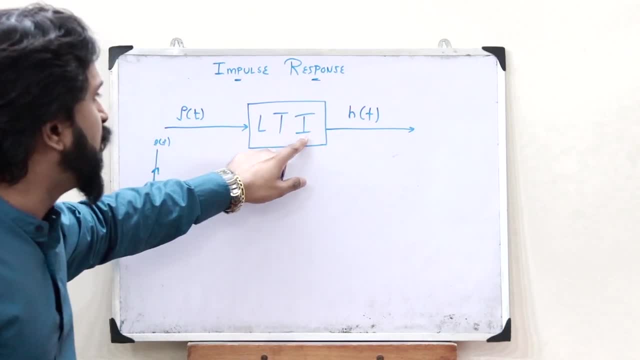 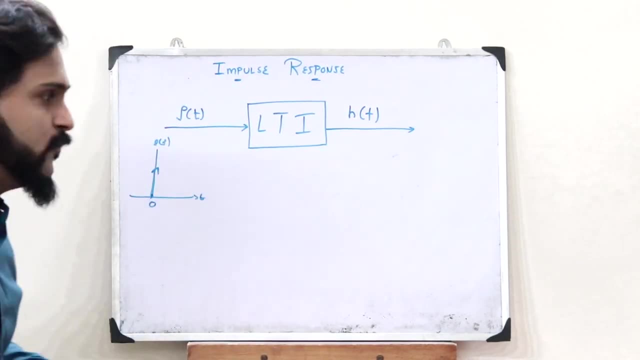 impulse response is the response of a control system when we give an impulse signal as an input to this particular LTI control system. Here the impulse response is represented by h of t. As simple as that, guys. this is simply what you refer to as an impulse response of a. 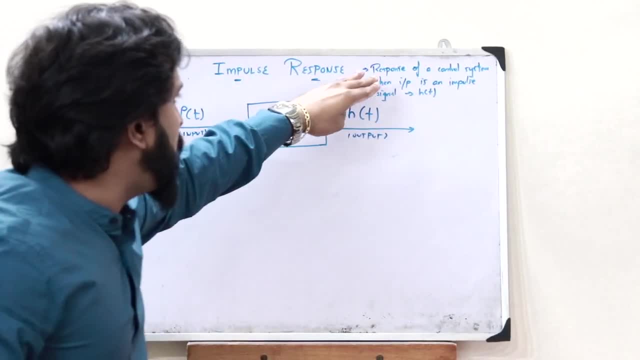 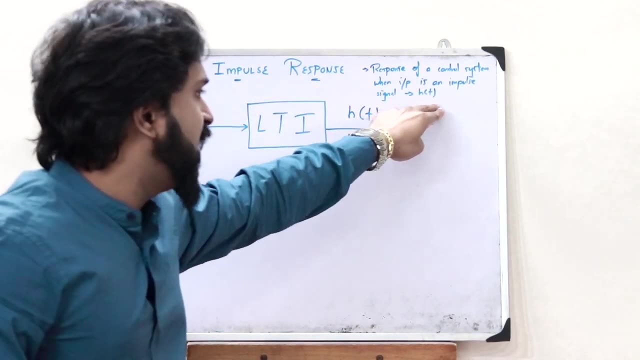 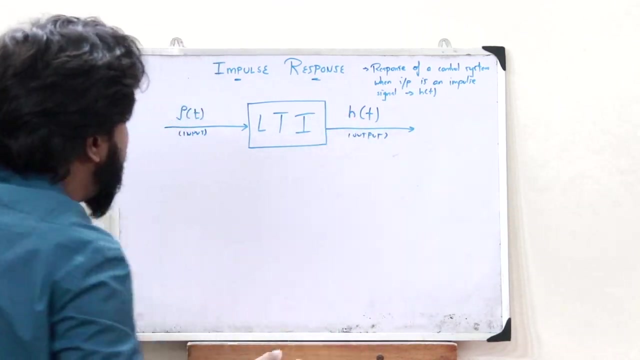 particular control system. So impulse response is a response of a control system when the input is an impulse signal and the impulse response is represented as h of t. So this is what you refer to as an impulse response. So this particular impulse response, h of t, is basically a characteristic. 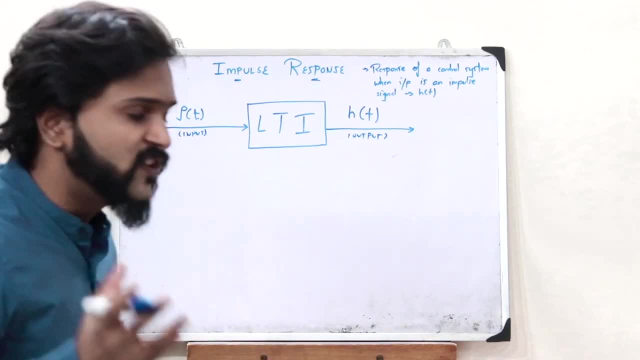 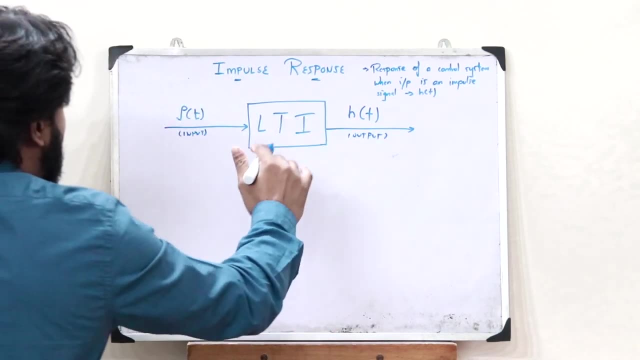 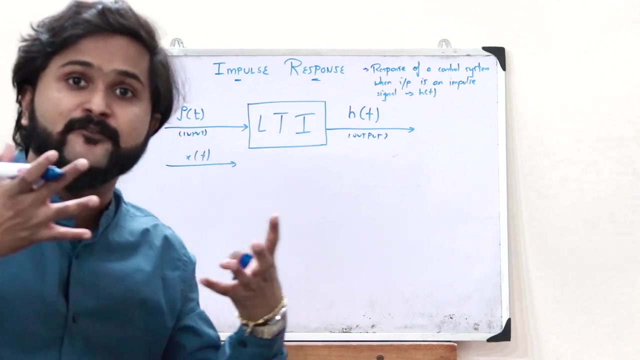 of this particular LTI system. Why is that? This is because if we know this particular impulse response- h of t- then when we give another input, say x of t, to this particular LTI system, with the help of this h of t, we can find what the value of the output we would get, which is y of t. 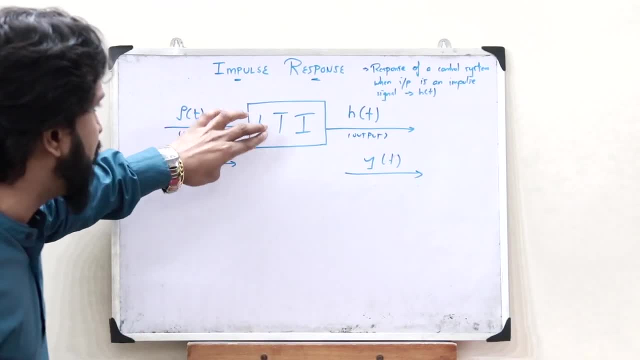 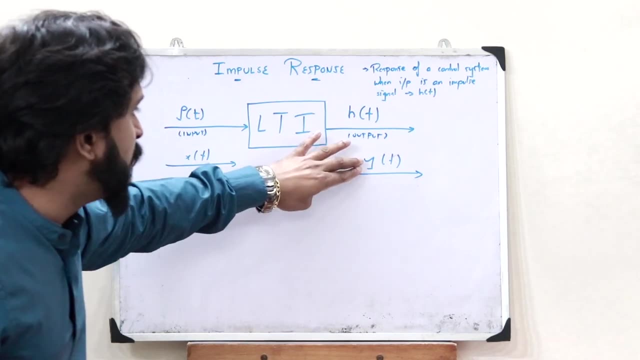 So that's it. Therefore, when we give a signal x of t to this particular LTI system, with the help of this particular impulse response, we can find out what the value of this particular output would be: y of t. for this particular input, x of t. But how is that? How do we find it? with the help of this. 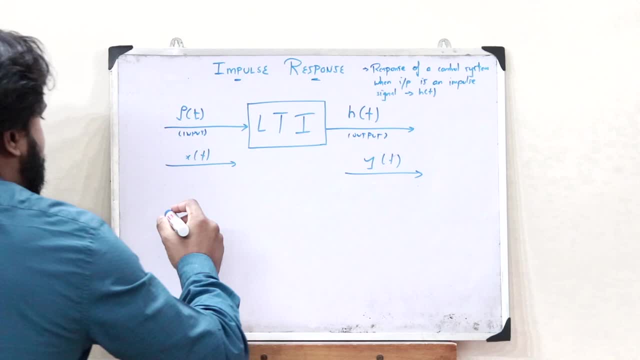 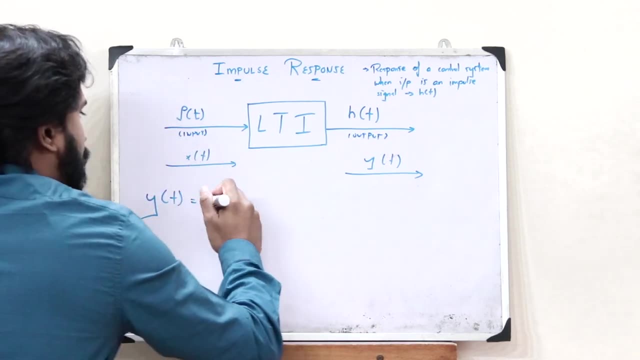 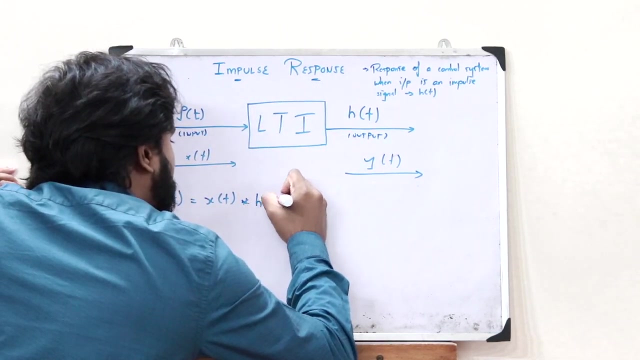 particular impulse response For that. here what we say is that the output y of t is obtained as the convolution of the input x of t with the particular impulse response h of t of that particular system. So that is how, with the help of this particular impulse response, 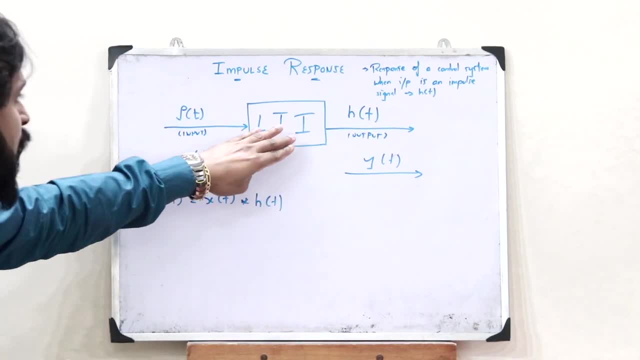 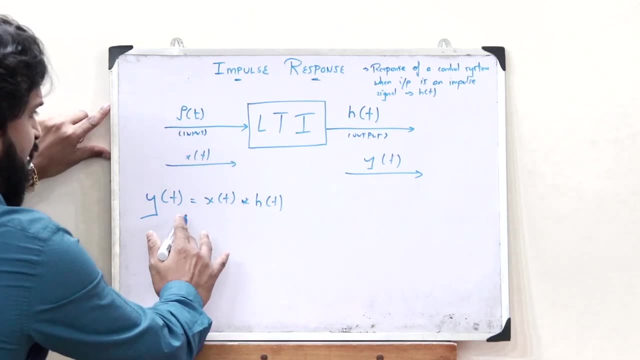 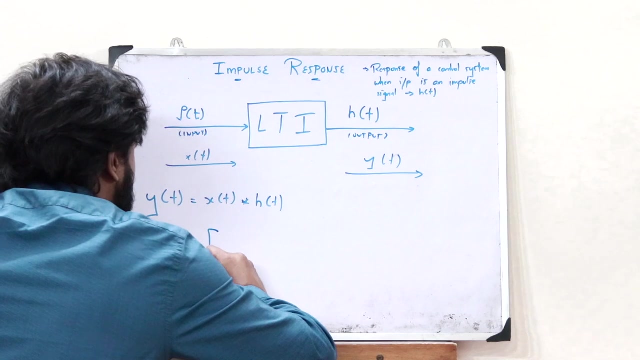 h of t. we can obtain the output from a particular control system when we give x of t as the input. So therefore, y of t is given as y of t is equal to x of t. convolution h of t. and now we know the formula for convolution: as y of t is equal to integral minus infinity, to infinity h of 2, into. 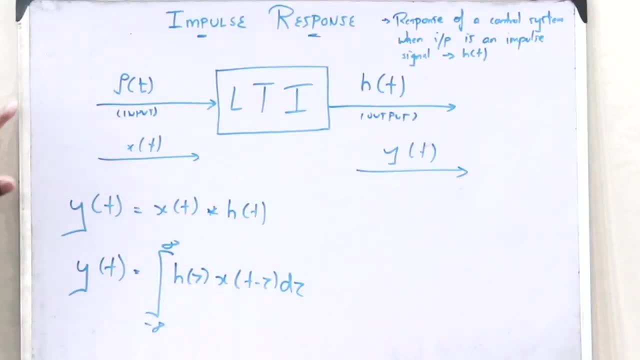 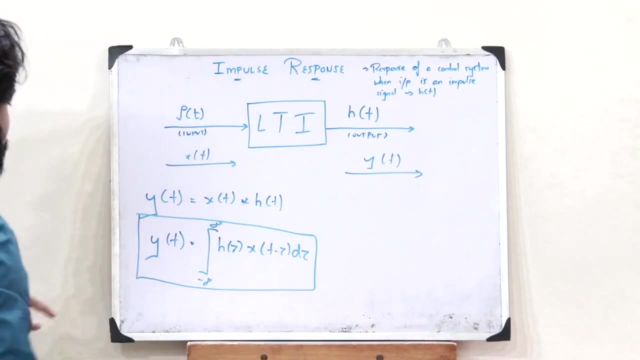 x of t. So that's how we can obtain the output from a particular control system when we give x of t as the input, t minus 2, d, 2, where here 2 is a dummy variable. So therefore this is the expression for the output y of t. 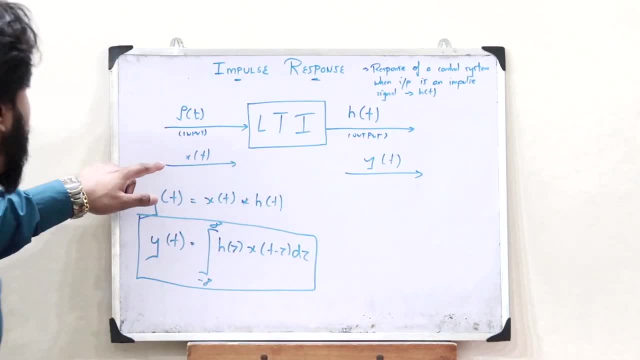 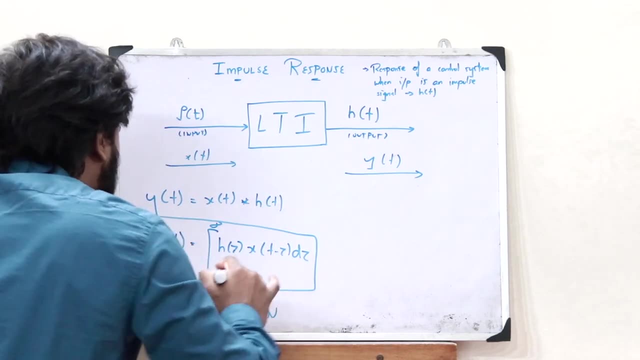 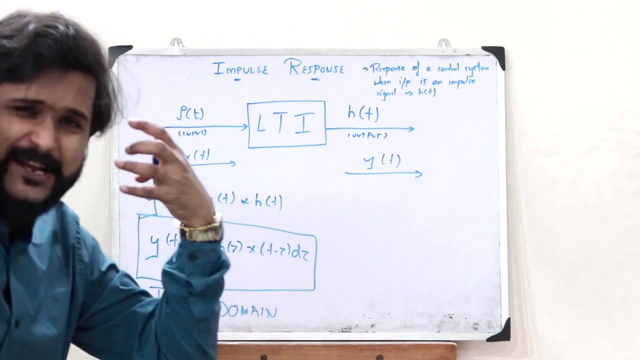 when we have a particular impulse response- h of t- and while we give an input, x of t, But but but this here is in the time domain. So here in the time domain, what we observe is that this is very complex. we have to find the integration of h of 2, x of t minus. this is very complex. 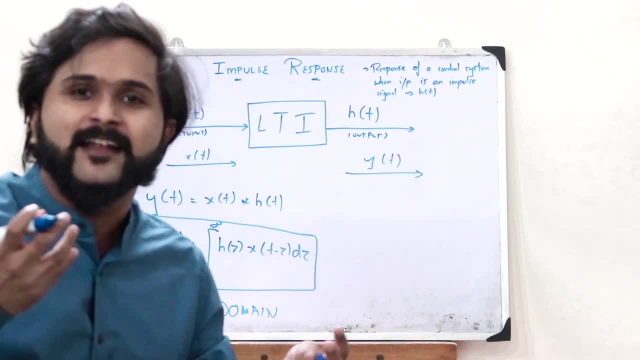 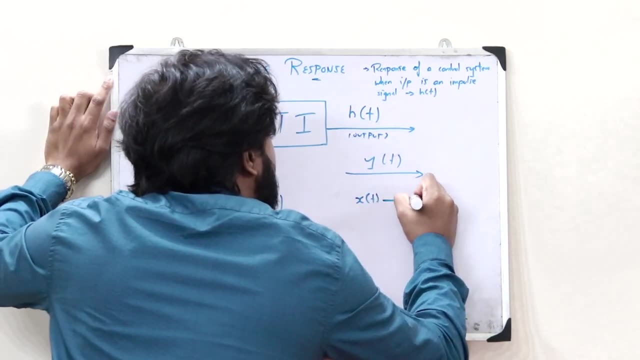 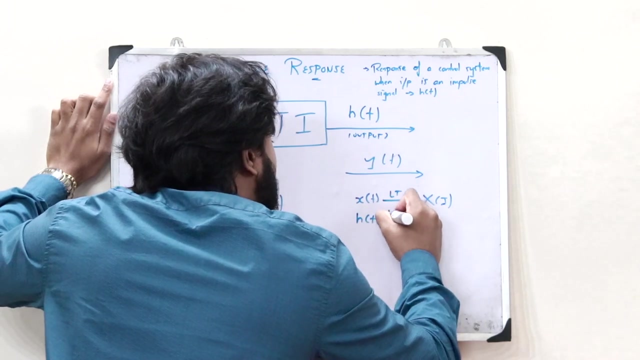 So, therefore, to simplify this, this is where the Laplace transform comes into play. So here, what we know is that the Laplace transform of x of t would give us x of s, and similarly, the Laplace transform of h of t would give us capital, h of s. That is, we are converting this from the time domain to 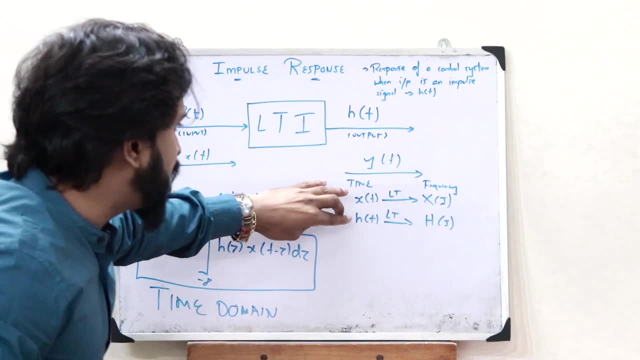 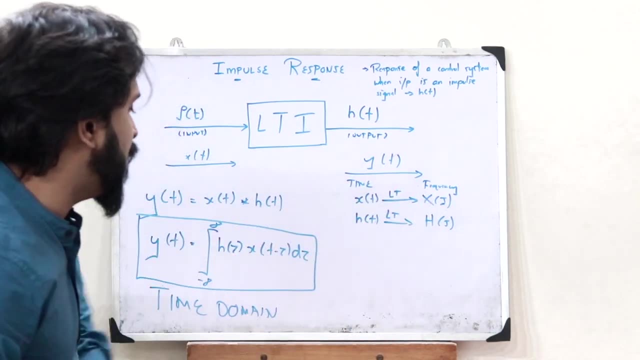 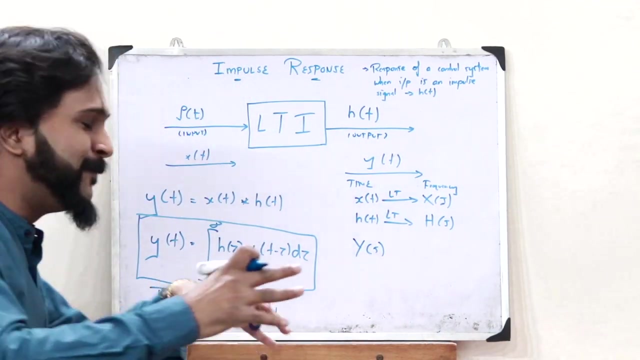 the frequency domain. So therefore, by taking the Laplace transform, we can convert x of t and h of t from the time domain to the frequency domain, which is x of s and h of s, and therefore the output y of s is obtained as the simple multiplication of x of s and h of s. So here: 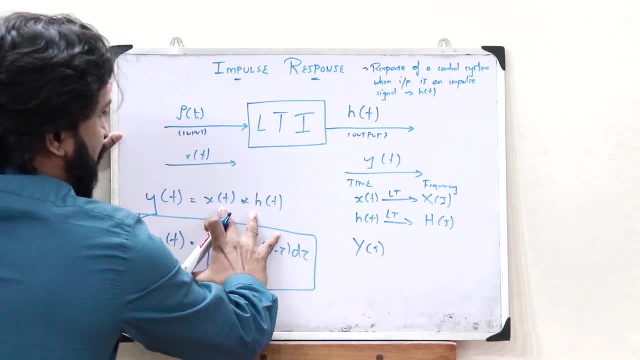 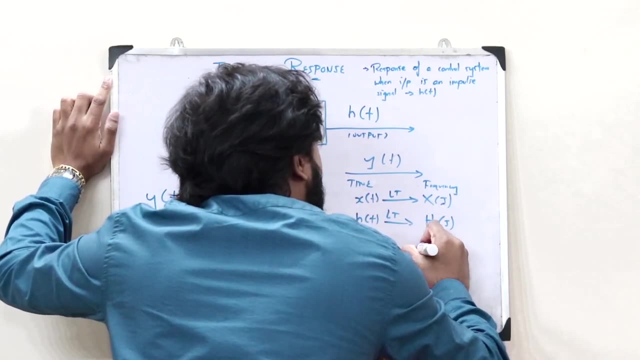 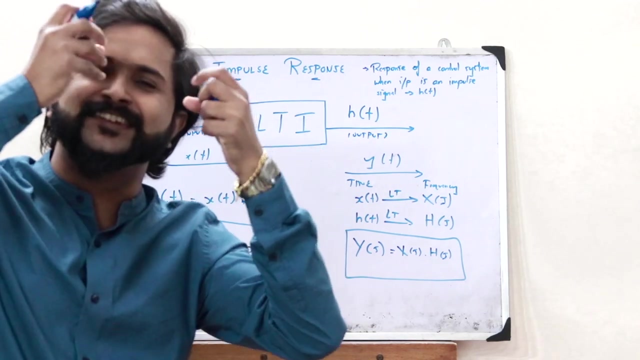 we are taking the convolution of x of t and h of t, but when these are converted into frequency domain, we simply just have to do the multiplication of x of s and h of s. So that is the beauty of the Laplace transform, That is, it just simplifies a whole lot of work for you. You don't have to sit and take the. 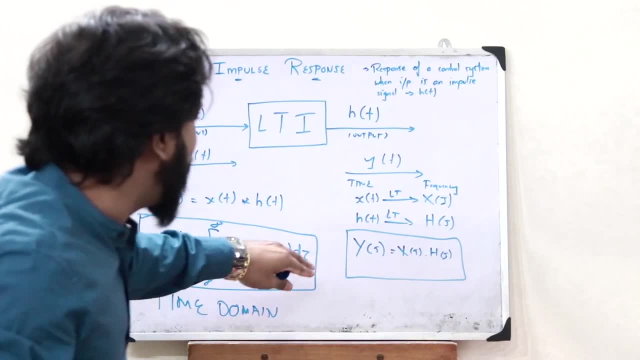 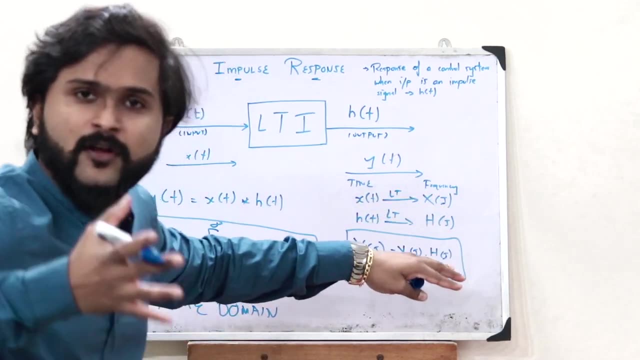 integration integral minus infinity to infinity. All those are eliminated. All you have to do is find the Laplace transform of x of t and h of t. convert it into the frequency domain. Once you have it, all you have to do is just simply multiply the Laplace transform. that is the frequency domain. 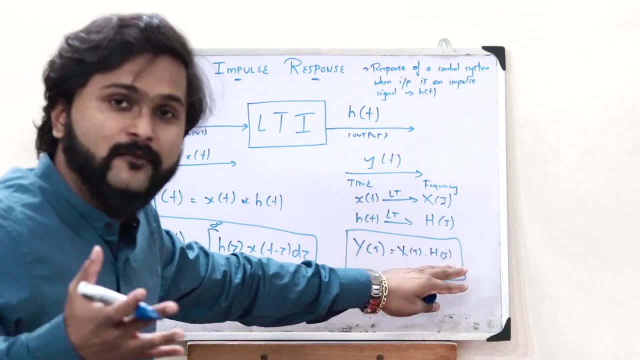 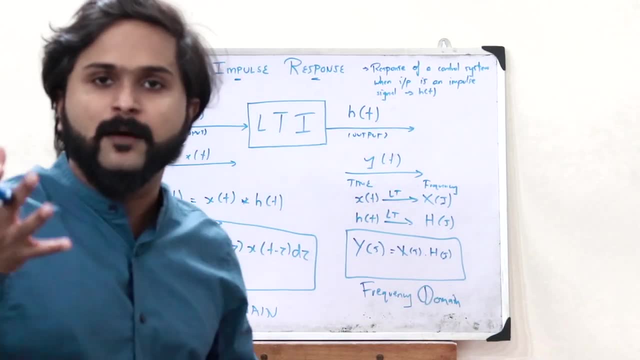 values x of s and h of s together. So thus we can obtain the value of the output in the frequency domain. So this property is what you are referred to as a convolution property of a Laplace transform, That is, if you have, say, two. 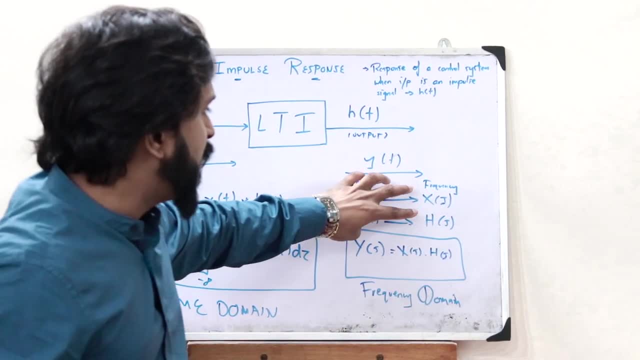 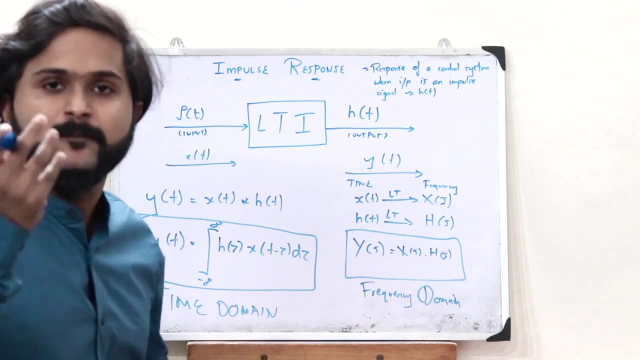 signals x of t and h of t in the time domain and the corresponding frequency domain values x of s and h of s. then the convolution of x of t and h of t is simply the algebraic multiplication of x of s and h of s. That's what we obtained over here. So this thus is: 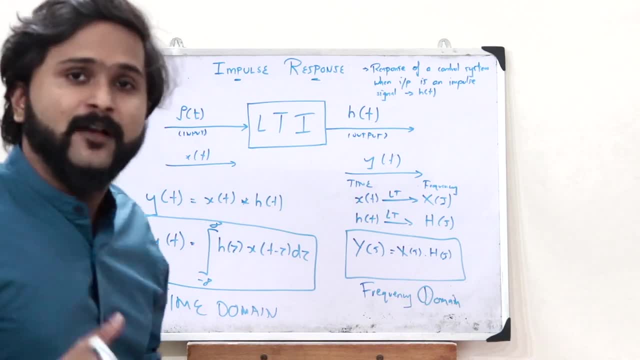 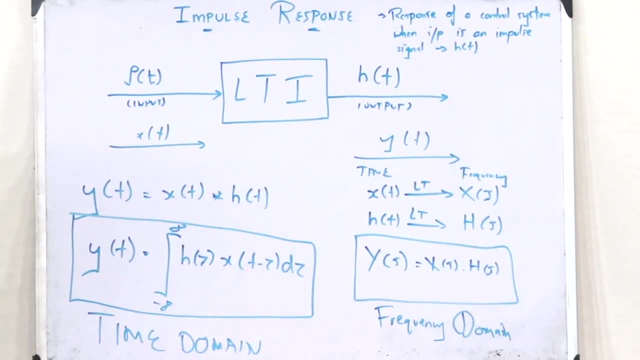 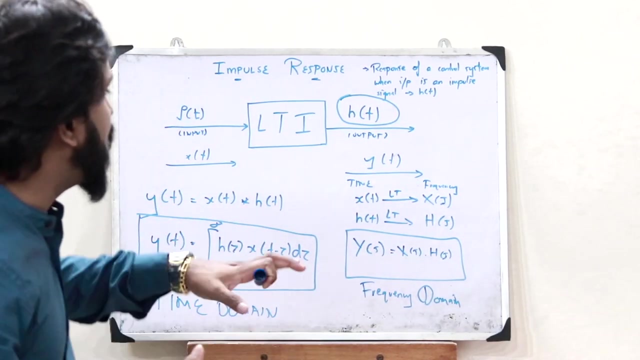 how we can find the output of a particular LTI system with the help of a particular impulse response. As simple as that, guys. there is nothing more to it. So, therefore, this thus is why we say that an impulse response is a characteristic of a particular 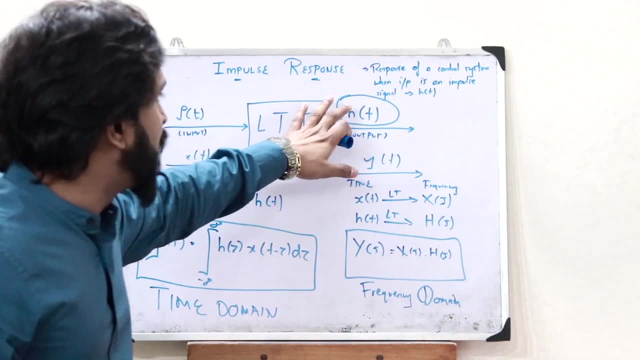 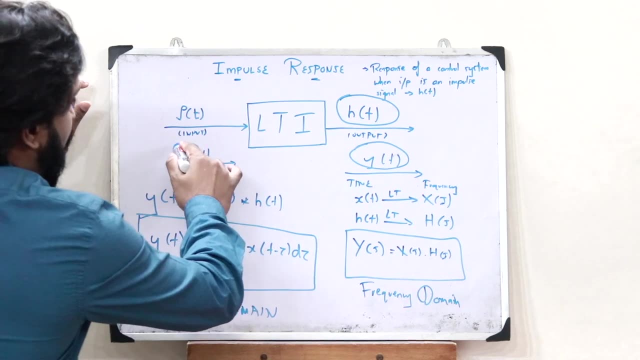 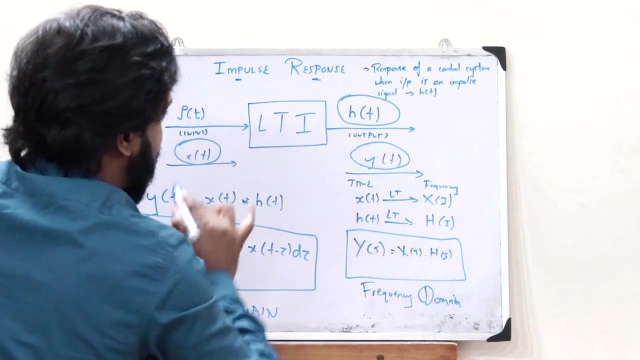 LTI control system because with the help of this particular impulse response, h of t, we can find the value of any output y of t when we give a particular input signal, x of t. This value of y of t is simply obtained as a convolution between x of t and h of t, That is in the time domain. but 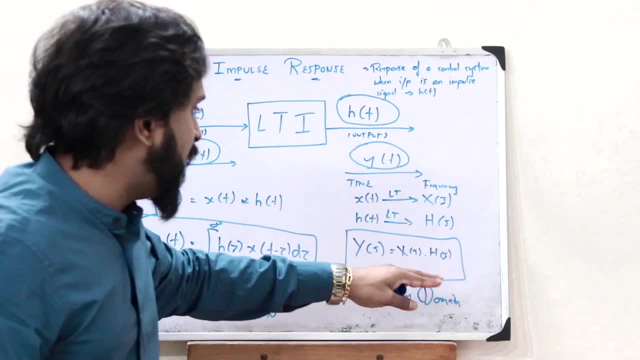 now, when we convert it to the frequency domain, we can find the value of any output y of t when we convert it to the frequency domain. All we have to do is now take the simple algebraic multiplication of these two in the frequency domain. As simple as that, guys. there is nothing. 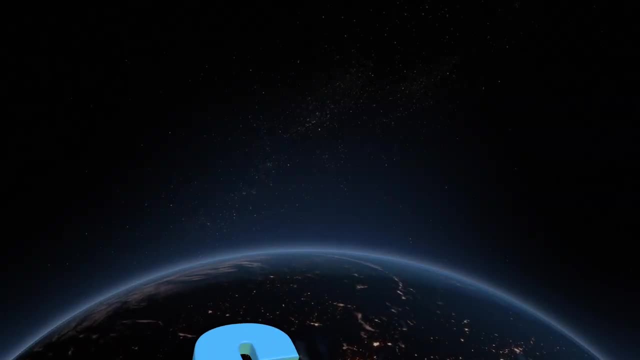 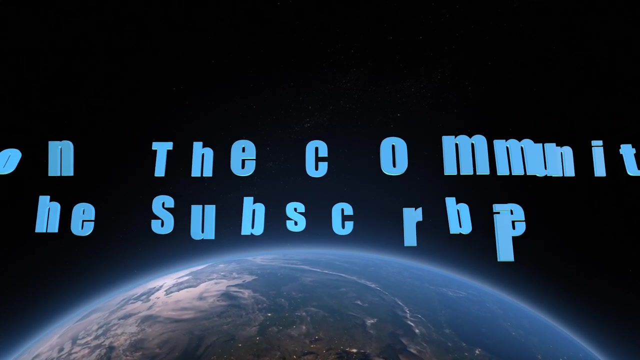 more to it. So I hope you guys now have a clear understanding of what you refer to as an impulse response of a particular LTI control system and if you guys found this video informative, please do hit the like button and join this community by hitting that subscribe button.